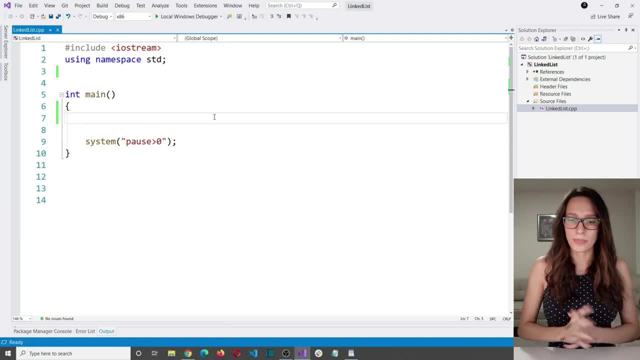 positioned in your memory, so all over the place. Now, your question might be okay, Saldina, but considering that Array stores elements one after the other, it's pretty easy to access those elements. but how do you access elements of a linked list? Well, the answer is that you need to. 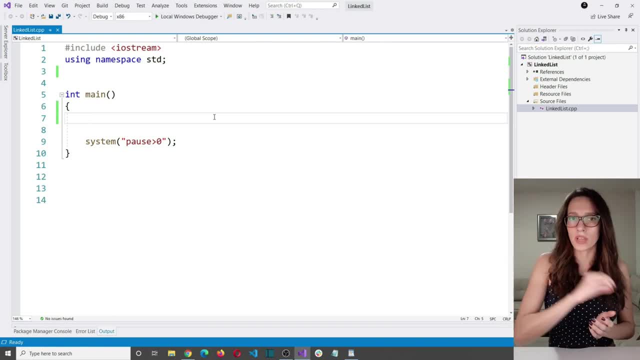 link the elements of a list in order to be able to access all of the elements. So, in order to explain this, let's use the example of a linked list that has four elements, For example. now, this here is going to be our first element, and that element is also known as head. Now this: 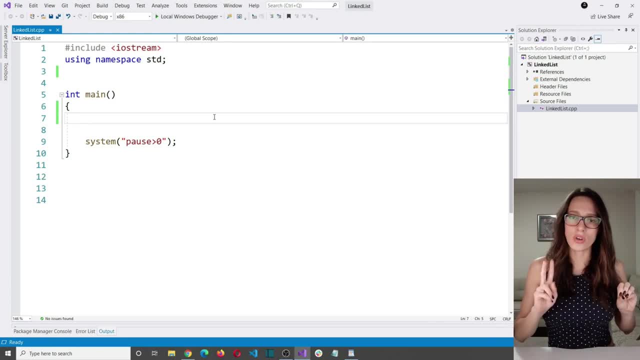 element here stores Two things. The first thing is going to be the value of that element, So let's say, for example, that will be a value of number one. and then, second thing that this head element stores is going to be the address of the next element. So it has a pointer to the second element. 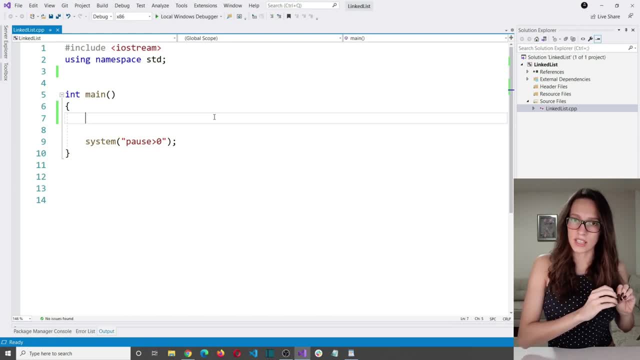 and it says: hey, in case that you are looking for the second element of this list, here is a pointer, Here is the address of that element. So here is our second element. Now, that second element also stores two things. The first one is going to be the value. So let's say: 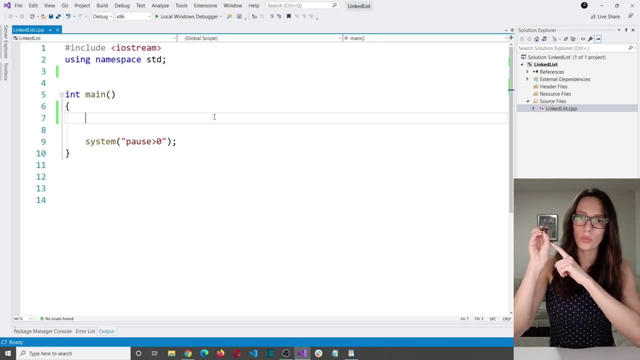 that will be number two, and then the second one will be the address of the third element, So it has a pointer to the next element. So here is the third element and then third element stores the value which is, for example, number three, and then it has the address of the next element. So 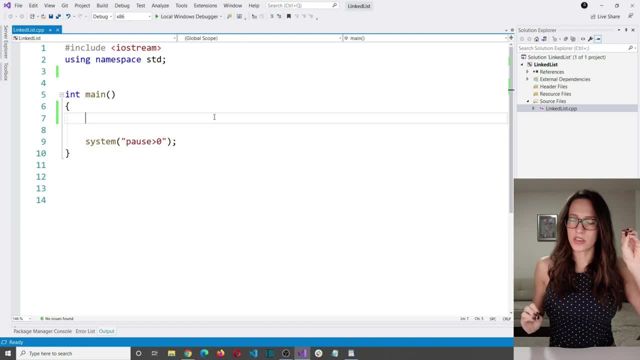 a pointer to the element number four, which is here, for example, and then this fourth element will also store the value, which is number four, for example, and then, instead of having pointer to the fifth element, it stores the value of null, because there is no fifth element. 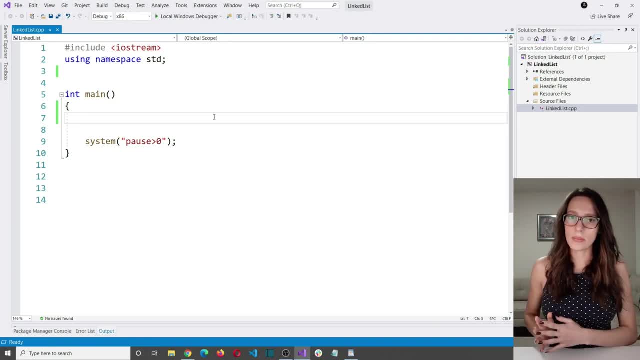 because this one is the last one. So the idea behind linked list is that each element stores two things. The first one is going to be the value of that element and then second thing is the pointer to the next element, and then the last element stores the value of that element. 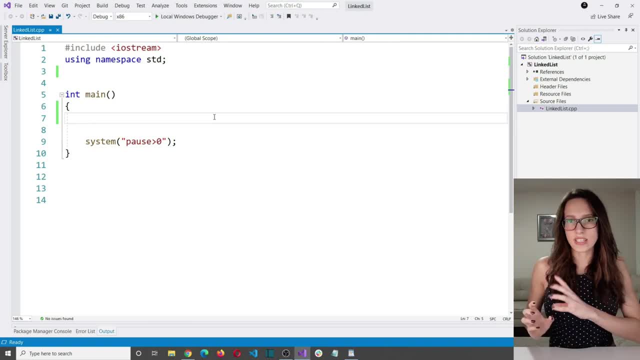 and then, instead of storing pointer to the next element, it stores null, because there is no next element, because that one is the last one. So what are some advantages and disadvantages of linked lists when compared with arrays? The biggest advantage is that arrays have fixed. 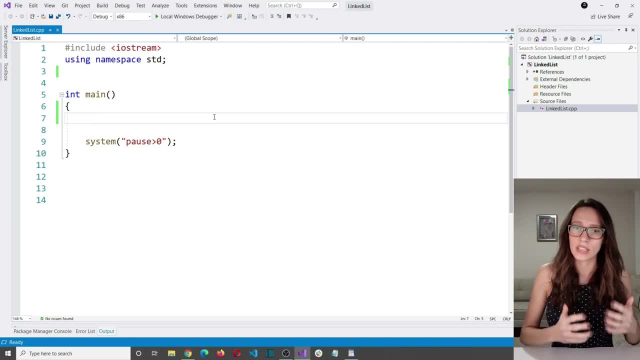 size and linked lists don't. Linked lists have dynamic size, which means when you create an array. when you create an array, you don't have to have a fixed size. So you don't have to have a fixed size to allocate memory for your array. It stays that size forever, which means that you cannot add. 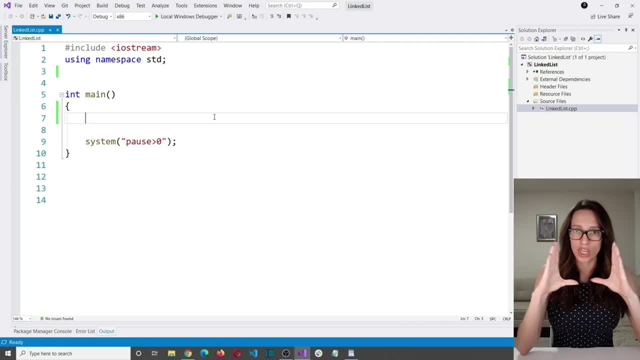 new elements, nor remove existing elements and change the size of that array. But in case of linked lists, you can always add new elements and remove existing elements. So that is the biggest advantage of linked lists when compared with arrays. Now, with this being said, there are some. 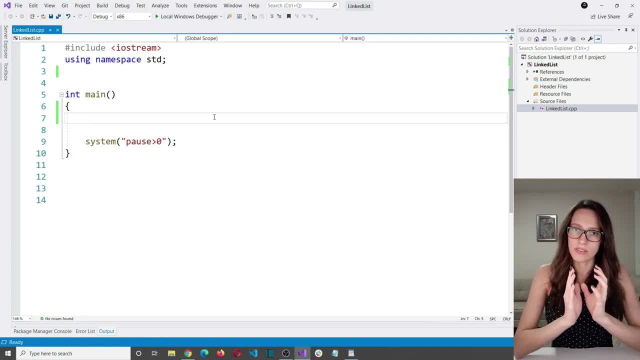 disadvantages as well. So let's get started, So let's get started, So let's get started. So the first disadvantage is that random access to the elements of a linked list is not allowed. What does this mean? Well, how will you access fourth element of your linked list, For example, can you? 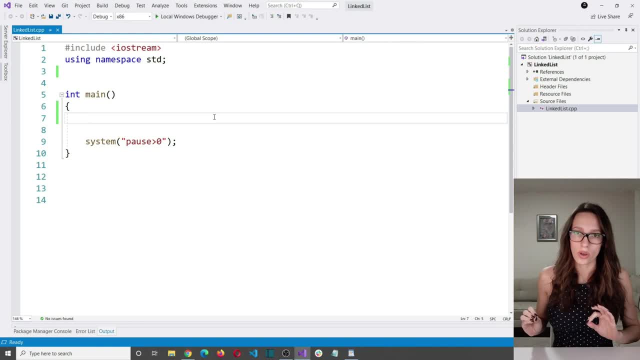 do that directly? The answer to that question is no. Why? Because you don't know where your fourth element is. because it can be anywhere in your memory, because elements are randomly positioned in your memory, So you can't access fourth element of your linked list, So you can't access fourth. 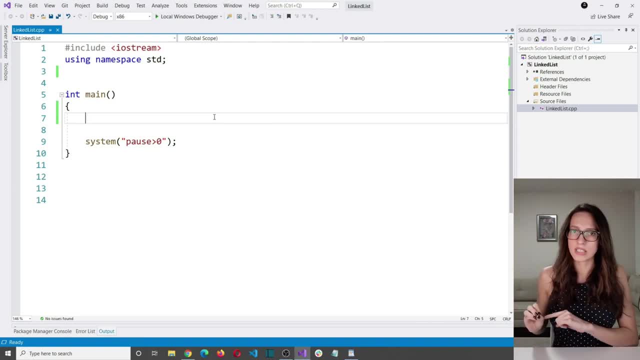 element of your linked list. So you can't access fourth element of your linked list. So who knows where the fourth element is? The answer is third element because it stores a pointer to the fourth element. And then who knows where the third element is? The second element: Who knows where? 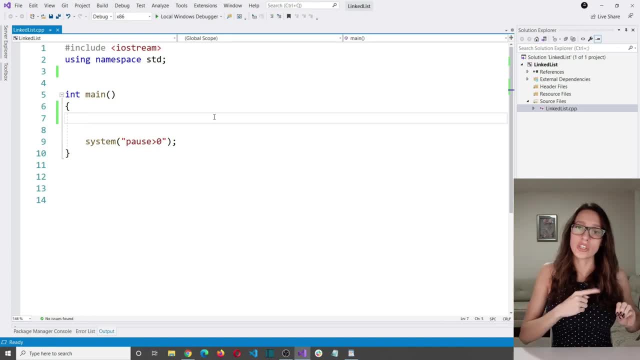 the second element is The first one, And you only know where your first element is. So you only know where your head element is, And then your head element has the pointer to the second one, and second one has the pointer to the third one, and third one to the fourth one. So you only know. 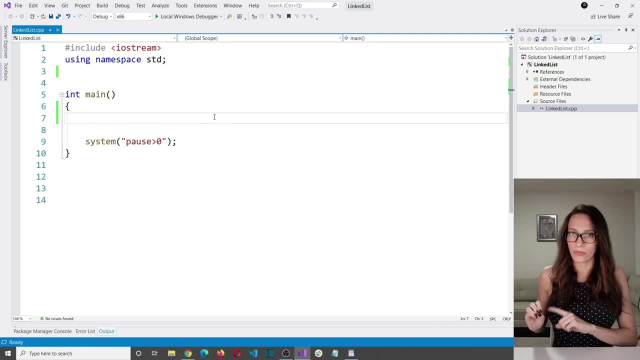 where the first element is and second one to the third one, and so on. So, in case that you want to access the fourth element, you need to traverse this path, And in case that you want to access the 400th element, or 4000th element, you need to traverse a very, very 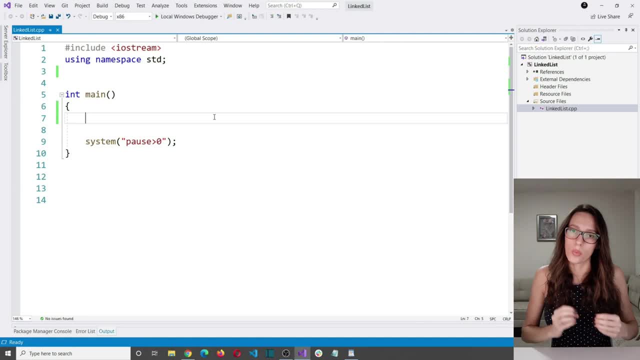 very long path. So that is one disadvantage of linked lists, Whereas an array that has a fixed size, and every array has a fixed size, the access to the elements can be direct because already know, hey, this is my array, And in order to access a fifth element, for example, I can use 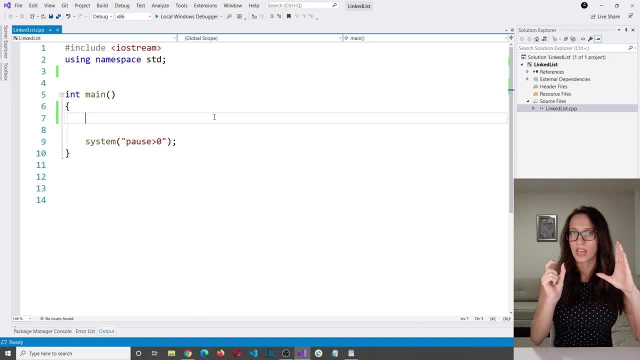 the name of the array and then the index of that fifth element, which is very, very quick. So that is going to be one disadvantage of linked lists. And then second disadvantage is that linked lists need more memory. Why? Well, as you already know, the element of an array stores only one thing. 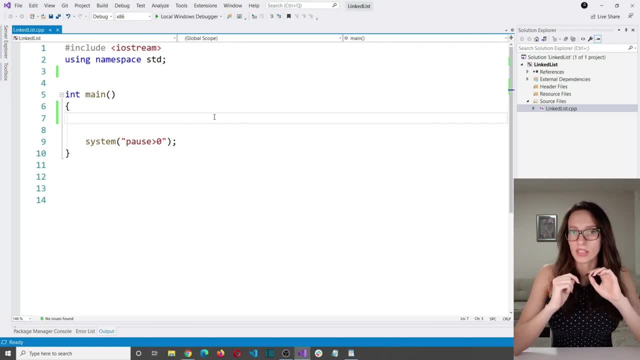 which is the value of that element. But the element of a linked list needs to store two things: the value of the element and then a pointer to the next element. So that is going to take more space inside your memory. So you need to do that for each element of your linked 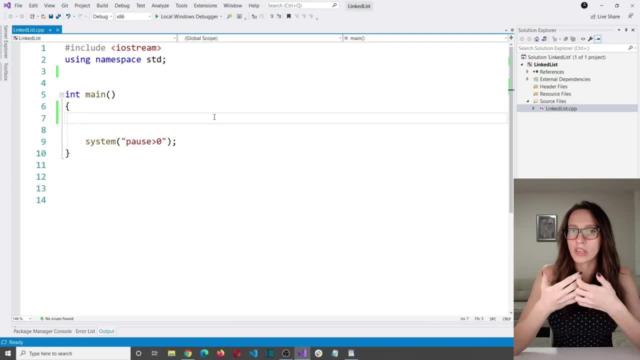 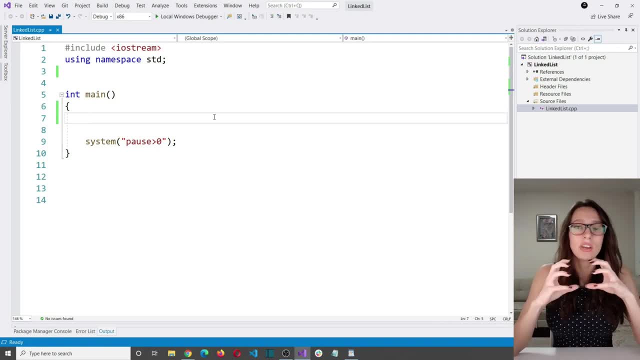 It's absolutely not Why? Well, because there is no such thing as better in general. You will need to choose what is better for each specific situation. So you will need to choose what is more important for your program, What is more important for the problem that you are trying? 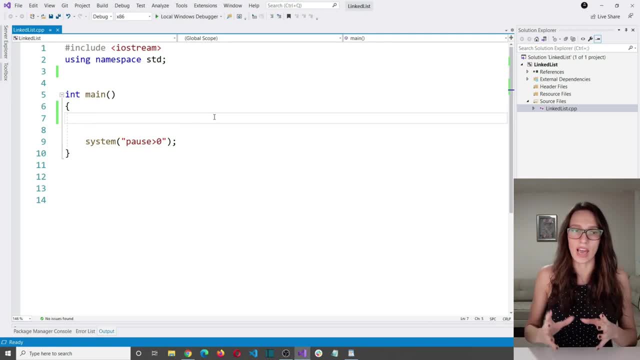 to solve. Is it more important for that collection to be able to access elements very fast Or will you be constantly adding new elements and removing existing elements And you need to take that decision and decide which one you will use: Either linked lists or. 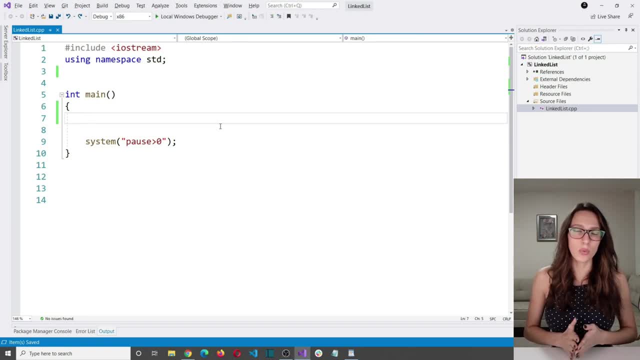 arrays. Another thing that I promised is that I will teach you how to implement a linked list using C++ programming language, And here I will implement a simple linked list that has only three elements, But that is going to be enough to demonstrate how linked lists work. 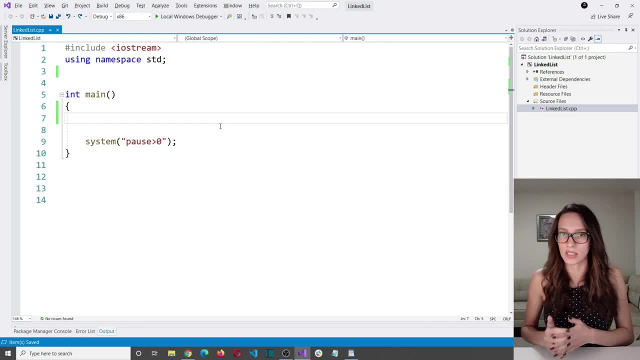 And then in the future I will be making more videos related to linked lists. So make sure to put all your questions in the comments down below so that I can read those questions by the time that I make my next video about linked lists. Now, another thing that I 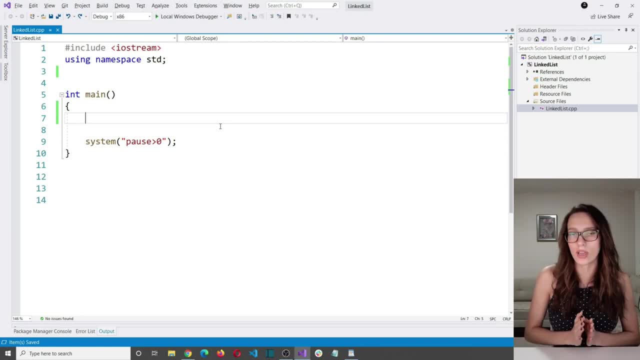 want to explain and remind you is that we said that each element of a linked list is going to consist of two parts. The first part is going to be the value of that element And then the second part is going to be a pointer to the next element. So this means: 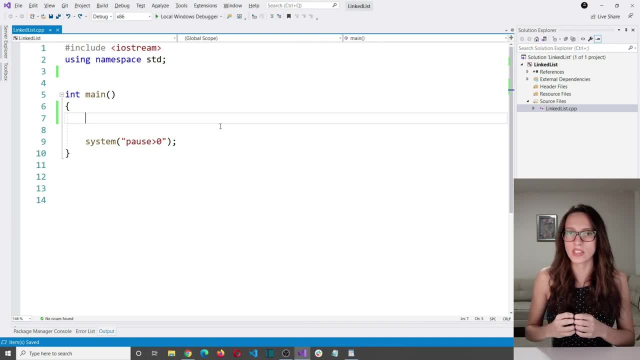 that you cannot represent an element of a linked list with a built-in data type, But you need to create your own user-defined data type in order to represent an element of a linked list. Now, I already made videos related to classes and structures And I will link a video related. 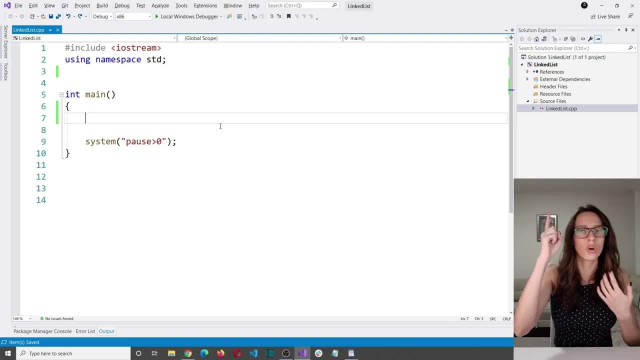 to classes here, So make sure to watch that video in case that you don't understand what are user-defined data types. And then as well in the description I will link both videos about classes and structures. So here we will be using a class which is a user-defined data type in order to 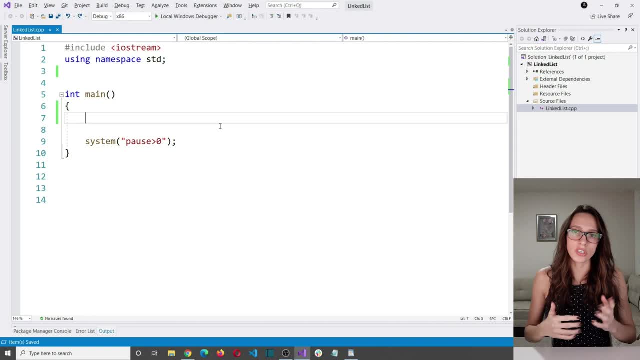 represent One element of a linked list. So, in order to name this class, you can use the name Element, But what is used more often is the name Node. So Node is an element of a linked list. So that is exactly what I'm going to do. I'm going to create: 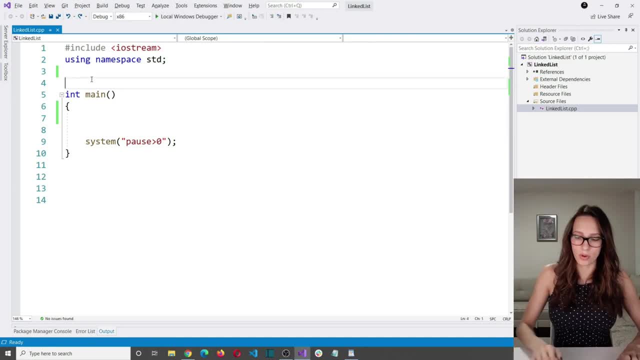 node. so let's do that. so here i am going to say class and then let's name my class node, as i said. okay, and here inside this class, i want to put two parts of each node which are the value of the node, and then a pointer to the next node, so a pointer to the next element. so let's say, for example, that 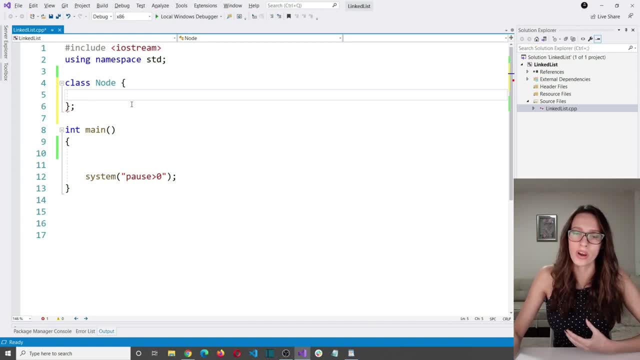 each element, so each node of our linked list will store an integer value and a pointer to the next element. so i'm going to say int value. so this is going to be the first part, and then the second part will be a pointer to the next node. so node, pointer, and let's call it next like this: now one. 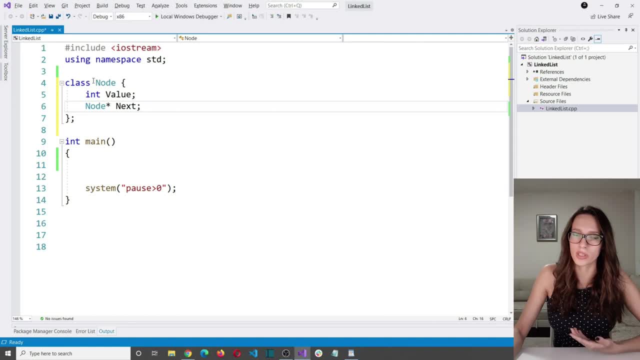 very important thing that you will not know if you are not familiar with classes is that all of the members of a class are private by default, which means that you will not be able to access them outside of your class, and in order to solve that problem, you need to use public access modifier. so i'm going to say here: 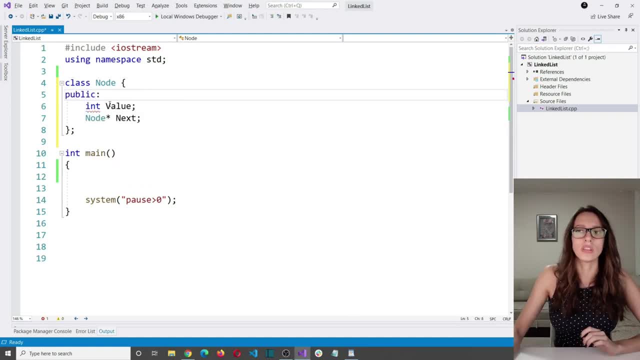 public like this: now, these elements, after adding this public access modifier, will be public, which means they will be accessible outside of this class, here and again. if you are not familiar with this, make sure to watch my full course. my playlist related to object-oriented programming, where i talk about classes and access modifiers. 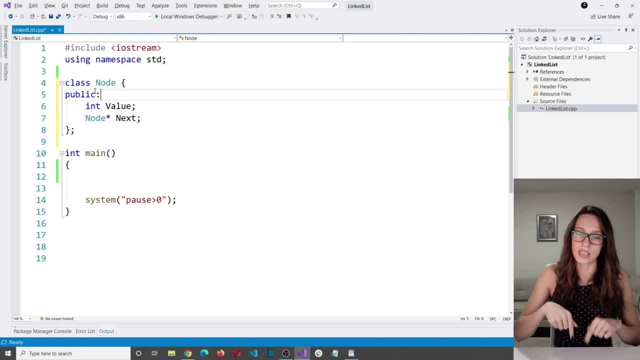 and many more things, and i will link that playlist here and in the description of this video as well. so with this, we have created a class called node, which is a user-defined type which is called node, and that represents one element of a linked list. so what i want to do now is i want to create three. 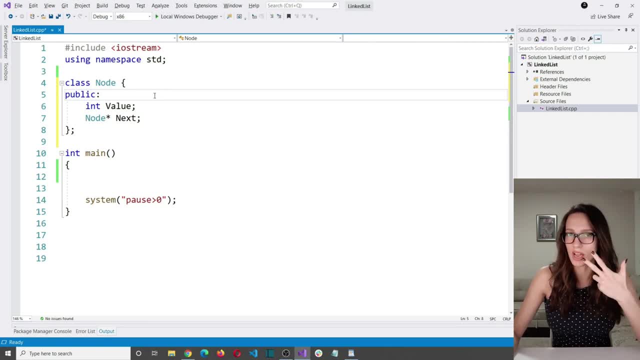 elements, because we said that our linked list will have three elements, so let's do that here in our main function. i want to create a pointer to the first element, which is the first element, which is going to be node pointer, and i'm going to call that element head like this: you can use the 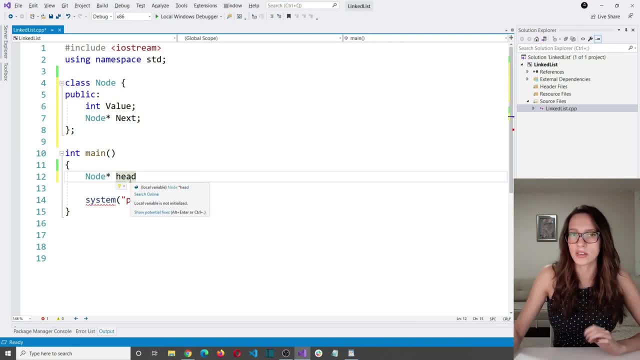 name first, if you want, but this is pretty standard naming convention. so i'm going to use the name head, because if another developer comes and tries to read your code and he sees the name head, he will know: hey, this is the first element of a linked list. so this is why you should also try to use 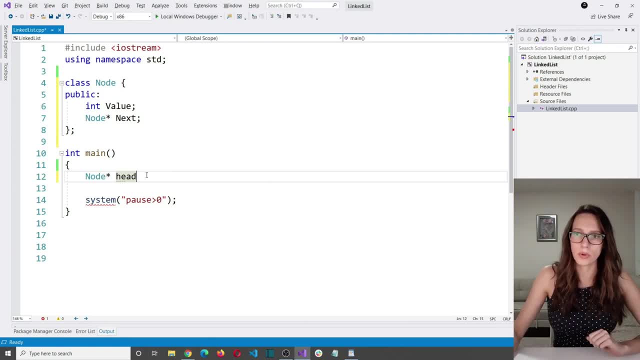 these standardized naming conventions. so i'm going to say that my head will be equal to new node like this, and i still have not assigned any values. i have just allocated the space for my first node and then, considering that this list will have two more elements, let's create those two. so i'm going to copy this line of code and then my second. 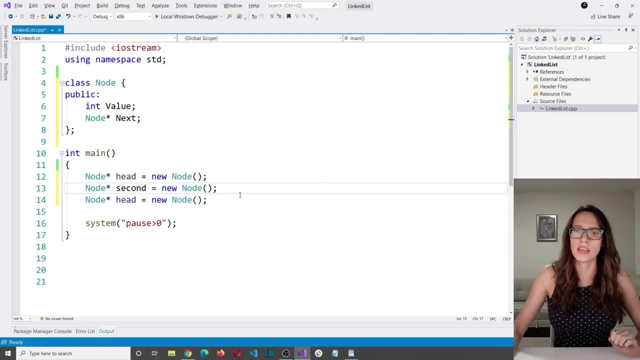 node will be called second, like this. and then let's call the third node third, like this. perfect. so with this i have created three pointers to three nodes: head, second and third. and i still have not assigned any values, so i still have not initialized the values of the value of each node. 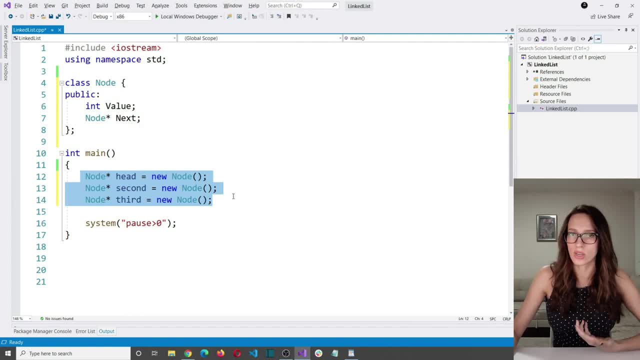 and then pointer to the next node. so now i'm going to do that. but first i want to say if you are not familiar with pointers and if you don't understand what are pointers, i have a full playlist where i explain what are pointers and how to work with pointers and i will link that playlist. 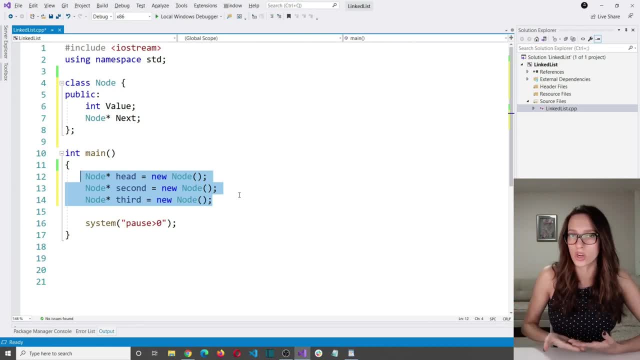 here and in the description of this video, in case that you want to watch that and understand this in more detail. so what i want to do next is i want to assign, for each one of these nodes, i want to assign the value and the pointer to the next element. so here i'm going to say that my head 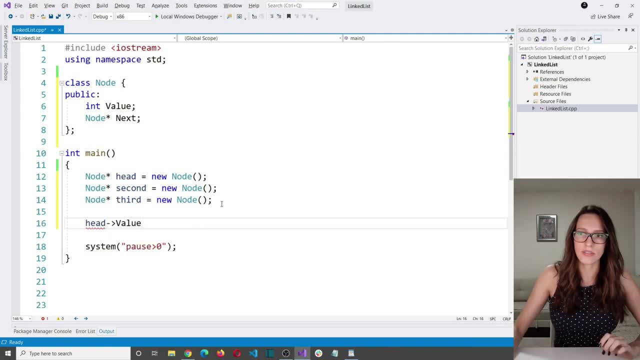 node will inside its value property, it will store the value of one, so the value of our first node will be one, and this symbol is used when you are trying to access members of your class in case that you are using pointers, like we are here. so you use this symbol instead of dot symbol. so i'm going 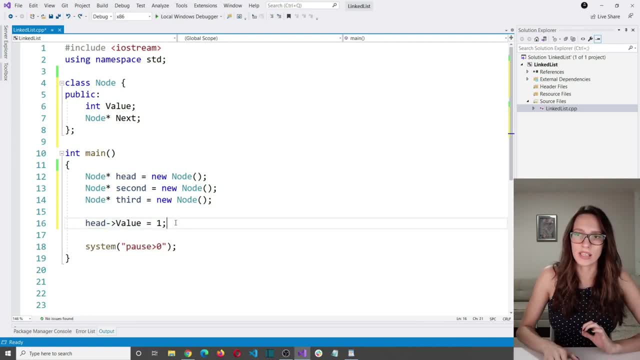 to return it to this symbol. okay, and then let's do this same thing for our second and third element. so i'm going to say that the second element value will be equal to two and then third element value will be equal to two, and then third element value will be equal to two and then third. 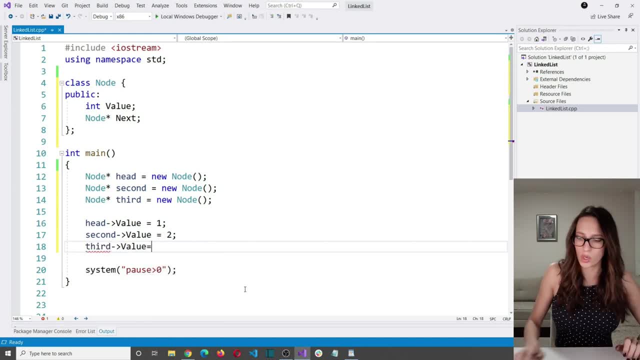 element, the value of that element will be equal to three, for example. now, with this, we have only assigned the values to these three elements, but we have still not linked the elements of our list, and that is very important step. so it is very important each time that you are creating a linked. 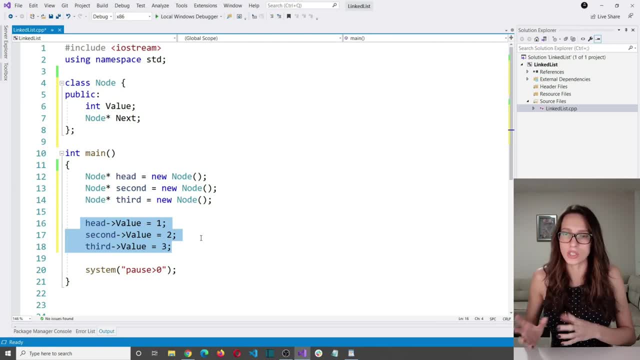 list to link all of the elements of that list. so how do you do that? well, let's do that first for our head element. so here i'm going to say that, i'm going to say that, i'm going to say that i'm going to my head element. the value of its next property is going to be this second element of the linked. 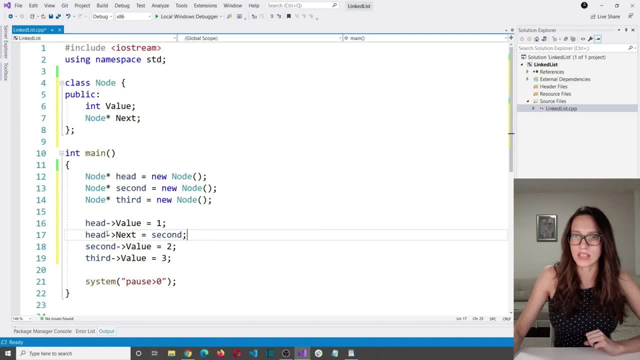 list like this. so now, what i'm saying is for this head element, the value of this next pointer here will be this pointer here. so our head element will point to the second element. so first points to the second and then second needs to point to the third and then third, considering 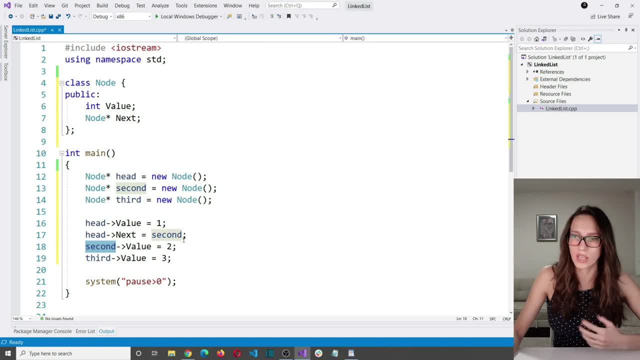 that it is going to be the last will point to null, so let's do that remaining part. so now i'm going to say second, next will be third. so now my second element is pointing to the third one, and then third element: considering that it is the last, as i already said, the value of its next pointer will be: 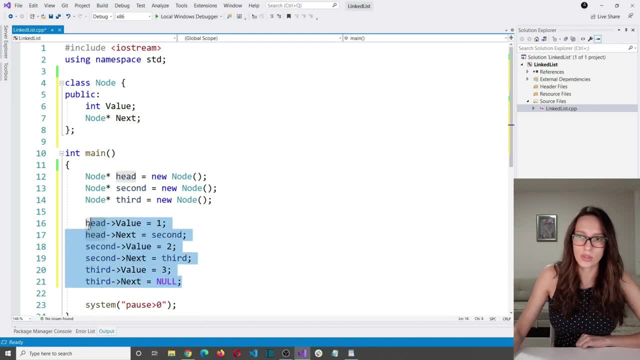 equal to null. okay, and now, with this here, we have successfully initialized the values of each element, and then we have also linked our list so that the first element points to the second, and then second points to the third, and then third points to null, because it is the last element of. 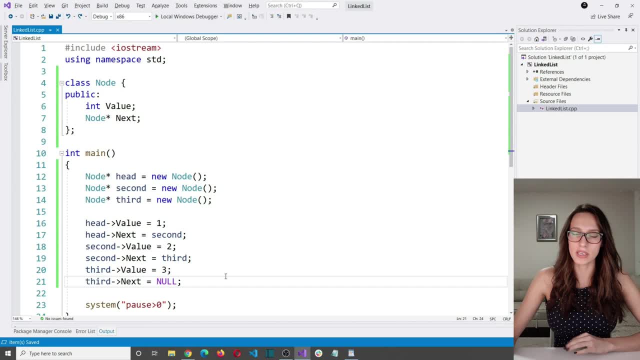 this linked list. so now your question might be okay, saltina, but how can i access the elements of each element when i want to have a list that is linked to the next element? so if i have a list, this list here, How can I print, for example, the elements of this list to my user? Well, let's do. 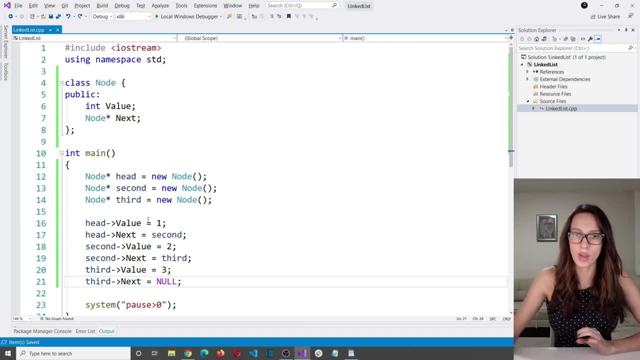 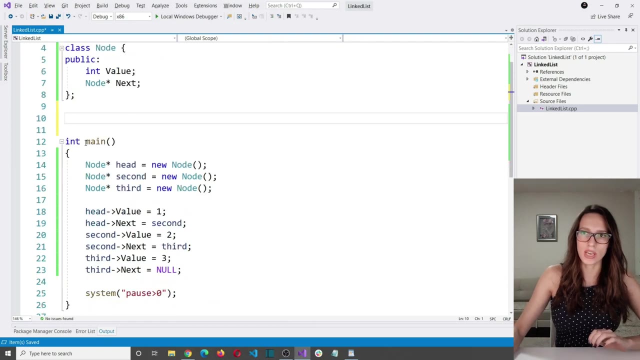 that. next, Let me show you how you can access and write out all of the elements of your list, And let's also create a function to do that, because I want to show you how you can pass a linked list to a function, So let's do that. here I am going to create a function of return, type, void And. 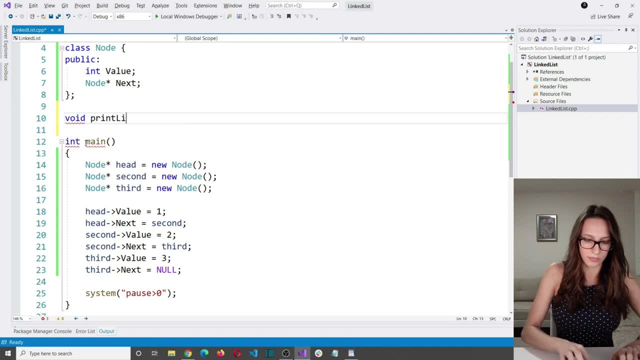 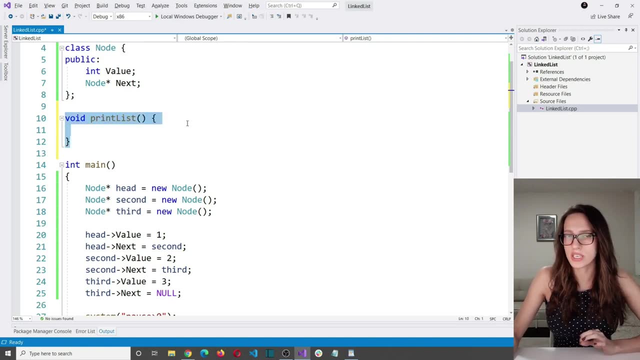 let's call that function- print list- like this. Okay, Now, what this function here needs to receive in order to be able to access and print all of the elements of this list? That is a question for you And that is a logical question. So make sure to pause the video and think about it, and 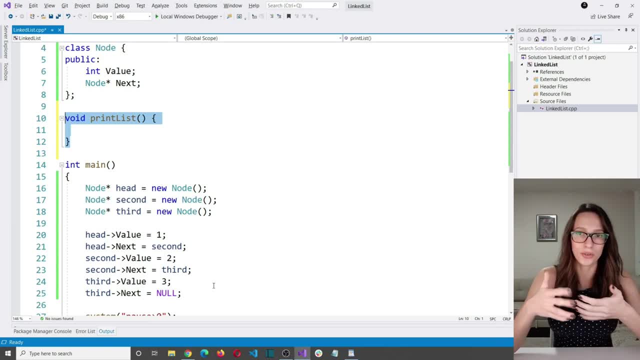 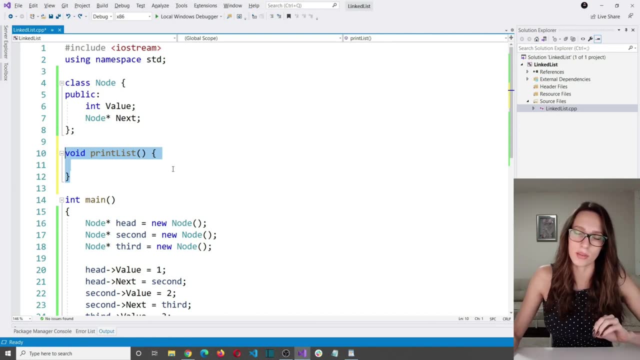 then write your answer in the comment section before you listen to my answer. So the answer is that it needs to receive all of the elements of your list. So let's call that function print list And let's say that it needs to receive the head element, which is the first element. Why? 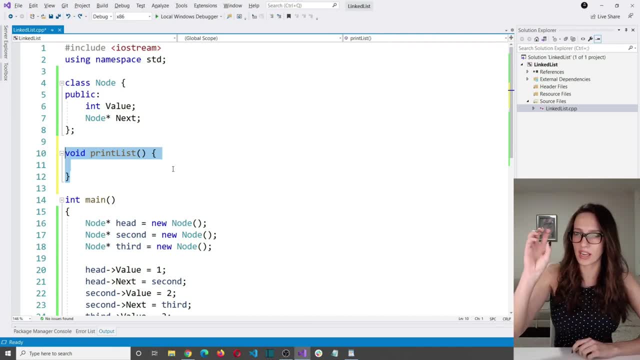 Well, because the first element has a pointer to the second element, and then second element has a pointer to the third element, And then third, considering that it is the last, it will not point to the next element because there is no next, but it will point to null. And when we come to null, 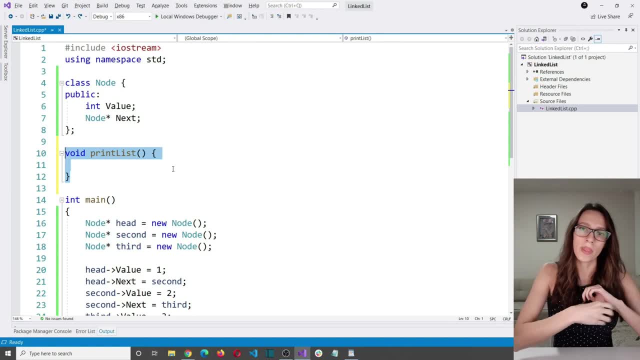 we will know. hey, this is the last element. So by passing the first element to this function here, we will be able to access and print all of the elements of this list. So let's go ahead and access all of the other elements of that list, no matter how many elements that list contains. 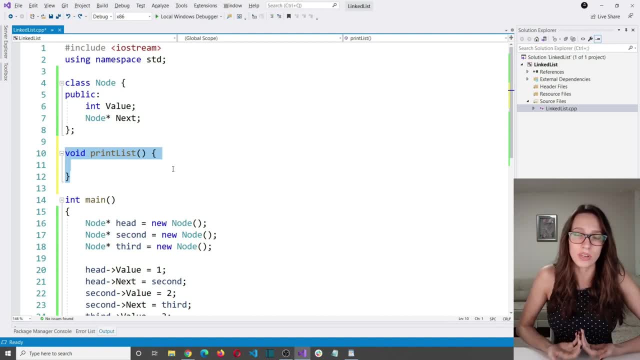 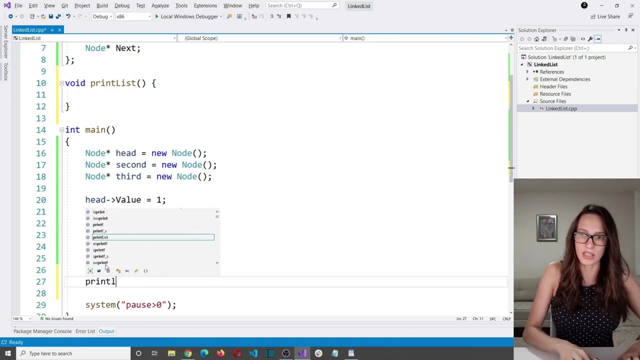 In this situation it is three, but you can have 300 elements or 3,000, or 300,000, depending on what kind of program you are building. So the invocation of this function here will look like this. So you will say print list and then you will pass to this function. 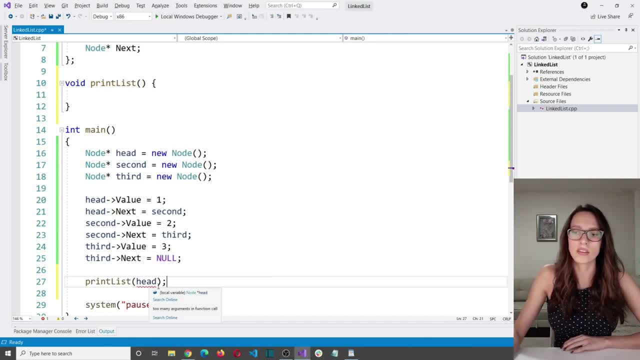 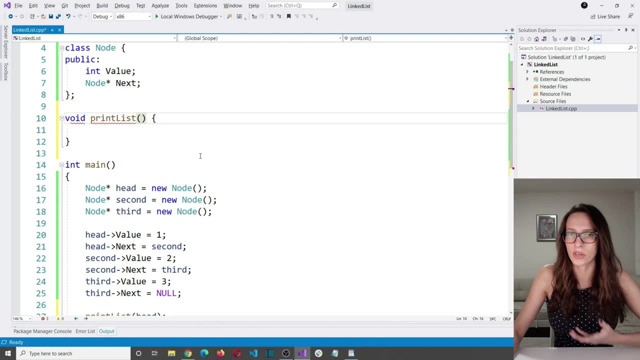 your head element like this, And then considering here that you are passing a node pointer, that means that here you need to receive a node pointer as well. So I'm going to say node pointer and I'm going to call this parameter n. Okay, Now what this function here needs to do is it needs to access all of the 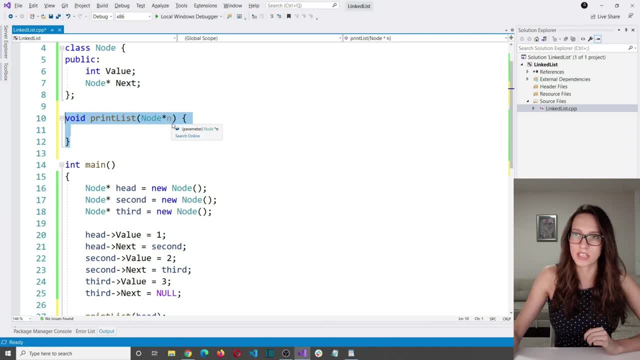 elements of the list, starting from this element here, and to print the values of those elements, to write those values. So, in order to do that, I'm going to use a while loop, So I'm going to say while, like this: 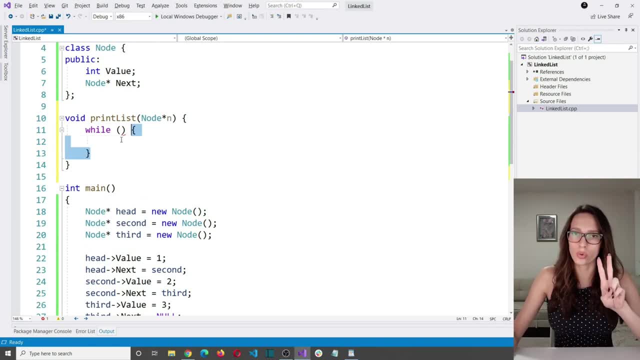 And then, inside this while loop, I will do two things. The first thing is going to be to print the value of the current element, And then the second thing will be to move to the next element. So let's do that. Let's say cout nvalue. 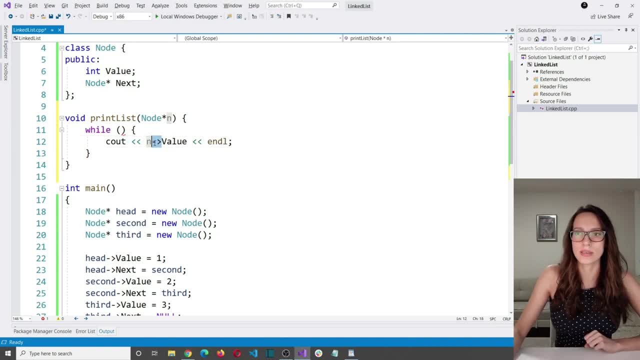 Okay, And let's add nline. And again, you use this symbol here to access elements of your class when you are using pointers. So this symbol is used instead of dot. even though I sometimes say dot, it is still this symbol here. And then the second part is going to be to move our node to. 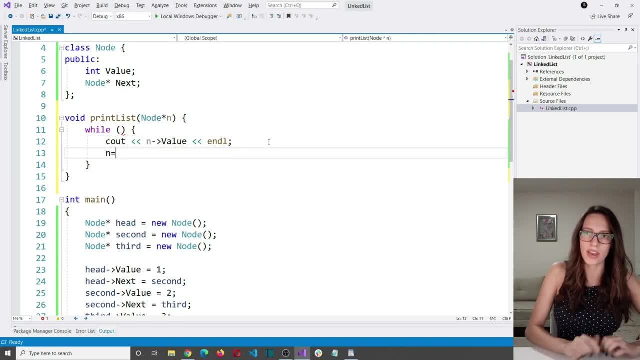 the next node. So I'm going to say that now my n will be equal to whatever our nnext is like this. So I'm going to do this, while our n is not equal to null. Perfect Now how this while loop is going. 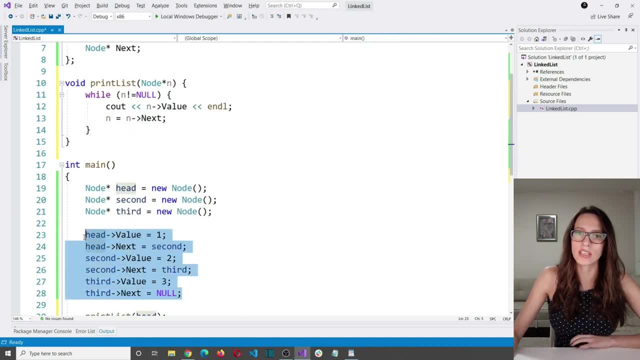 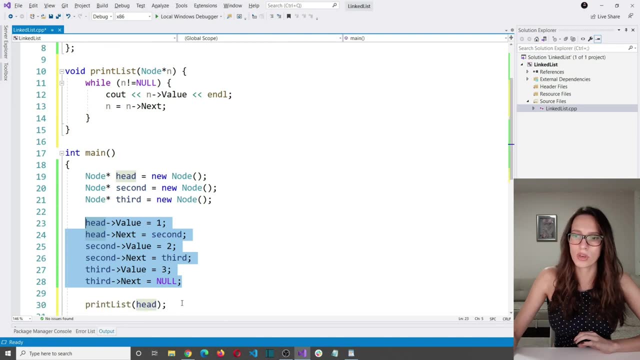 to behave in this situation, here, in the situation of a list that has three elements. Well, when we invoke this print list function, when we invoke it here, we are going to pass our head node to this print list function, which means that it will receive this element here. So we enter this element here. 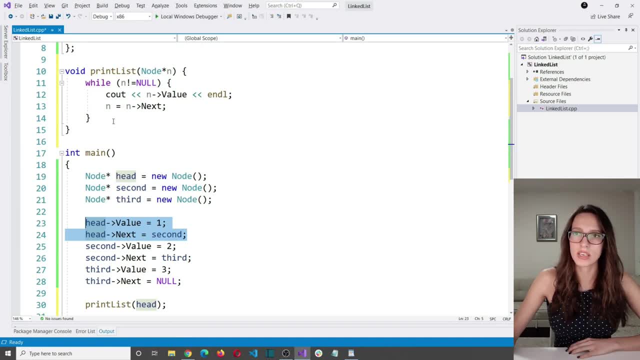 And the first thing that happens is it tries to go into a while loop. So it checks: is n different than null? Now, what is n? It is this head element. So is this different than null? The answer is yes, So we can enter inside this while loop, So we then print out n value which. 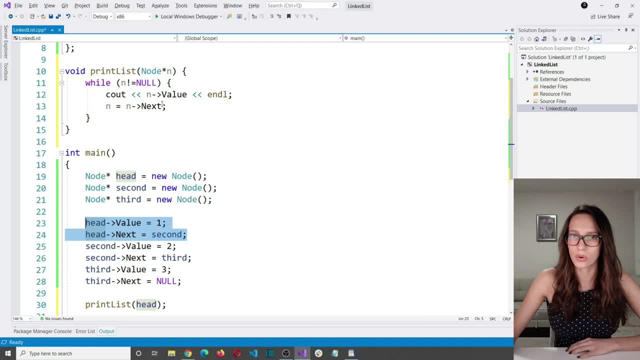 is one. And then we perform this second line of code here which says: now I'm going to move or to change the value of my n to whatever nnext is holding, And in this situation nnext or headnext is second element. So it is this one here. So it tries to go into a while loop again. 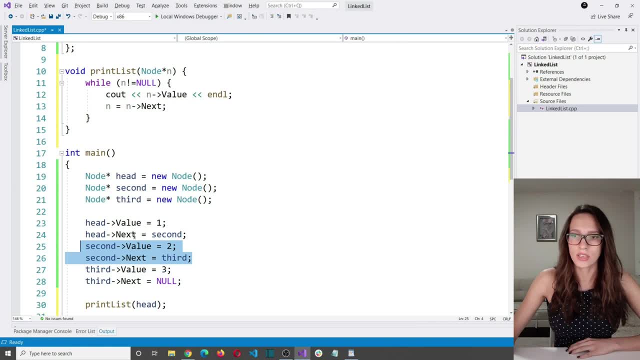 And then it checks: is n different than null? The answer is yes, This here is different than null. So we can go into our while loop again. So we write out again n value, which is two, As you can see here, And then we do this second line of code which says: now n is going to be whatever. 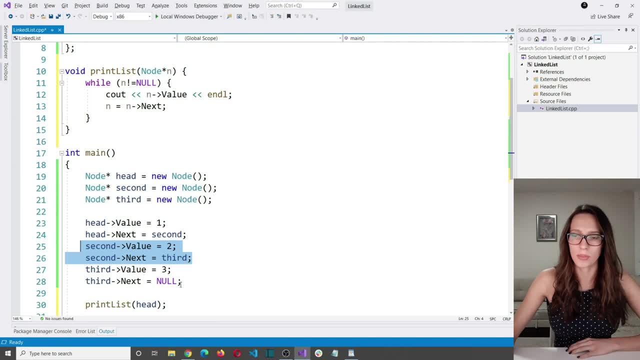 nnext is, And that is third element, which is this one here. And then it comes here and tries to enter in this while loop again. So it checks: is n different than null? Is this here different than null? The answer is yes. This third element is a legit element which has the value of three. 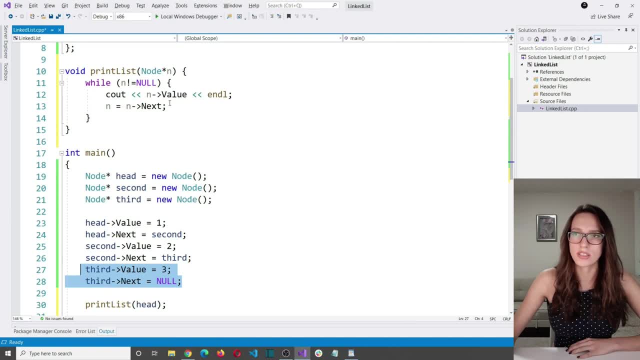 And it has this pointer to null. So we can enter inside this while loop again. So we print out the value of three here And then we move to this second line. And this second line of code does the following. It says now: my n will be whatever nnext is. And in this situation, 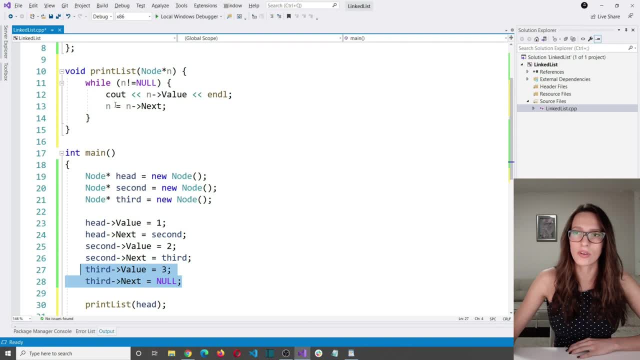 thirdnext is null. So that means that in this line of code our n becomes null. So when we try to enter this while loop again it checks: is null different than null? And the answer to that is no, they are equal. So that means that our n is null. So we print out the value of three here And then.